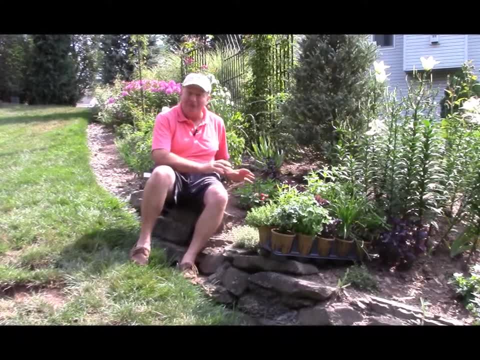 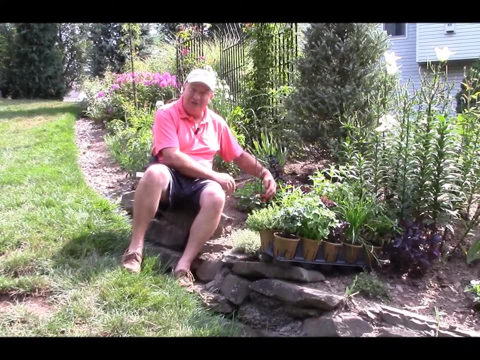 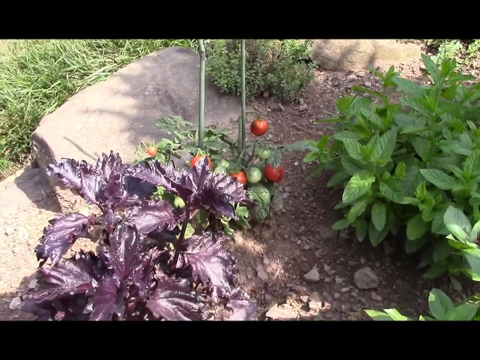 of planting and growing and picking some of the things that you'll be growing in the garden. There's nothing better than coming out and picking these little cherry tomatoes. These little cherry tomatoes are so sweet they can eat them right off the plant. and when they touch the leaves of this purple leaf basil- or perhaps touch the leaves on a 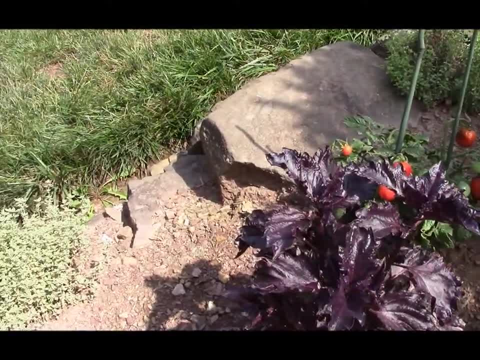 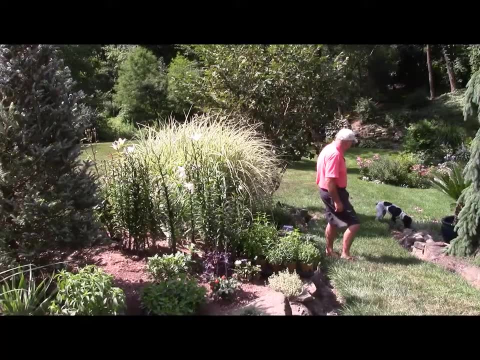 clump of mint, or even just brush against the leaves of lemon scented thyme, they'll be able to experience things that they wouldn't normally come across, And there's nothing better than coming out and picking these little cherry tomatoes. There's nothing better than coming out and picking these little cherry tomatoes. These little cherry tomatoes are so sweet they can eat them right off the plant. and when they touch the leaves of this purple leaf basil- or perhaps touch the leaves on a clump of mint, or even just brush against the leaves of lemon scented thyme- they'll be able to experience things that they wouldn't normally come across. 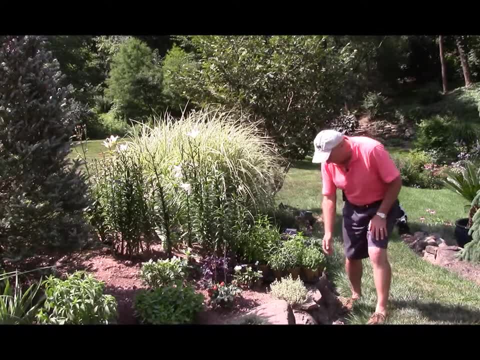 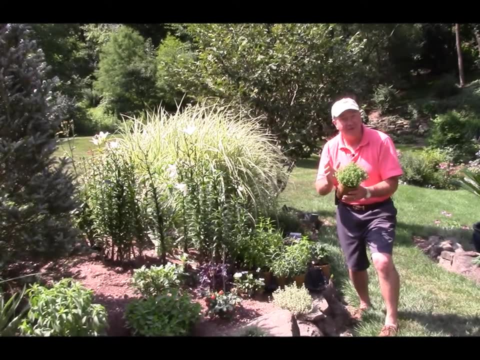 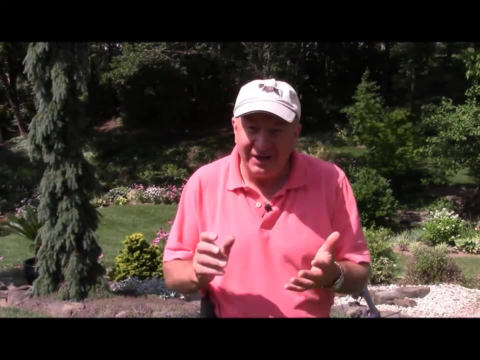 They like how these plants from Footprints Plants the edible line are nice, big, strong plants that when you plant them in the ground, grow away quickly and give quick results. Now, many years ago in fact, when I think about it now, it was several decades ago- I used to go and help my grandmother in her garden and that was the inspiration, the spark. 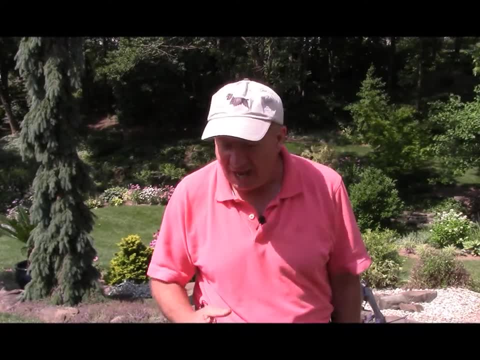 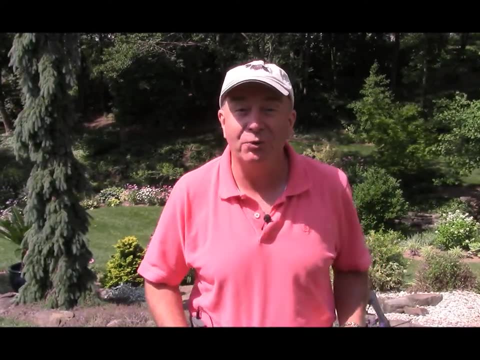 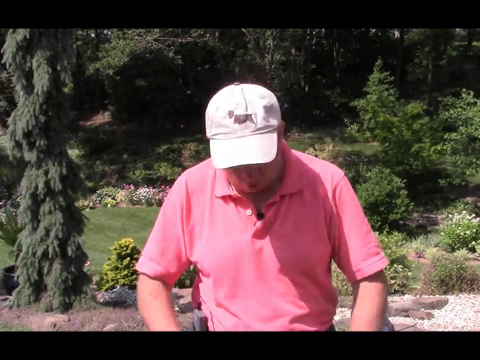 that got me interested in gardening and growing plants and led me on a very rewarding lifetime of growing and talking about plants and, of course, eating them too. So if you've got wee ones coming to visit- whether they be grandchildren, nieces and nephews or your own little ones- take them out into the garden and 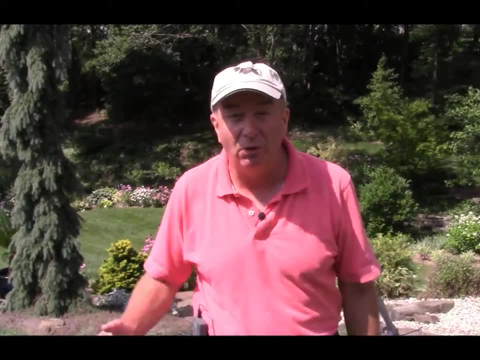 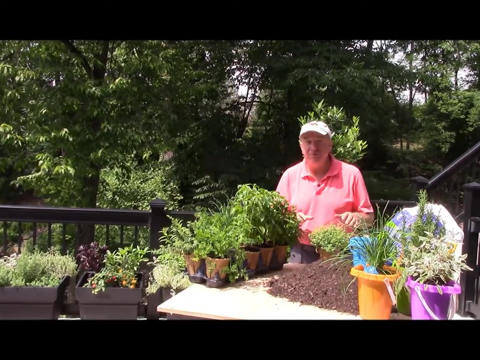 let them see something of what's to be done when they grow outdoors. It's good for them and, of course, it's very nutritious too. Now, of course, it's very important to make it both fun and interesting, and here's a little idea that I think you might. 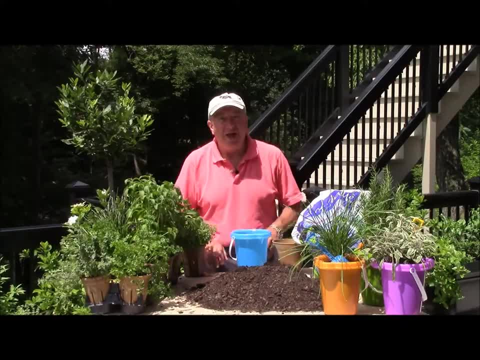 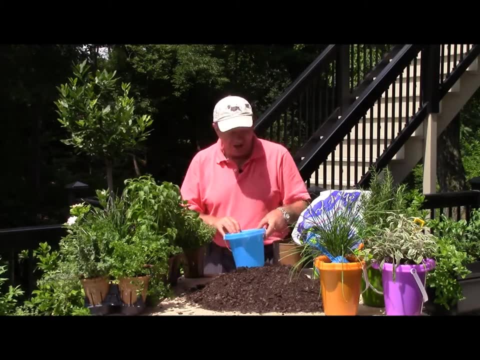 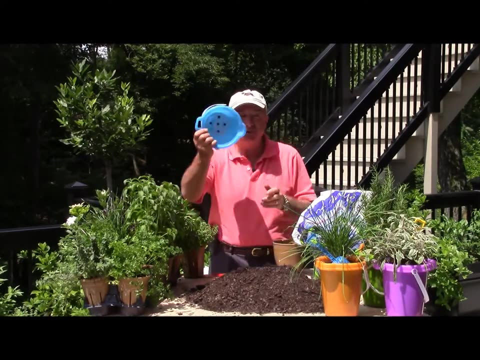 like to try, And that's growing them in a fun container. Now, it could be almost any sort of thing, even an old shoe or a boot. In this case, what I'm using, as you see, is a little bucket and spade. Children love this sort of thing. If you use them, just make sure to have holes in the bottom. 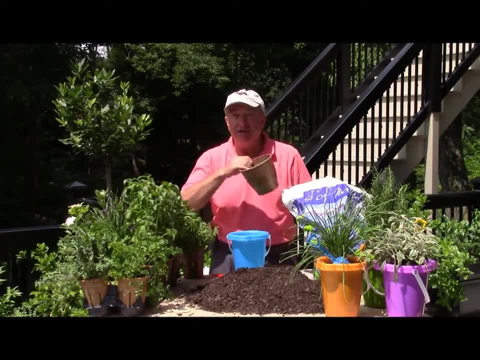 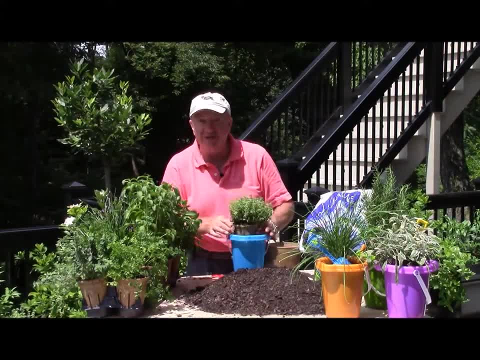 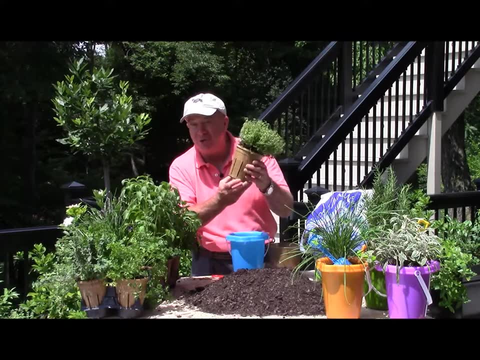 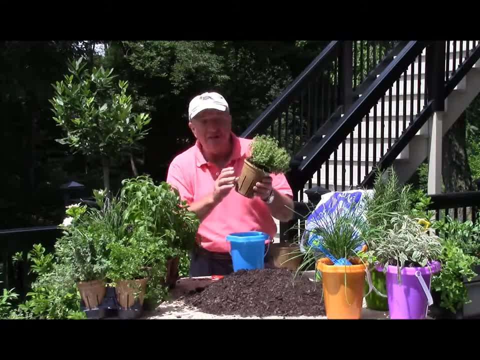 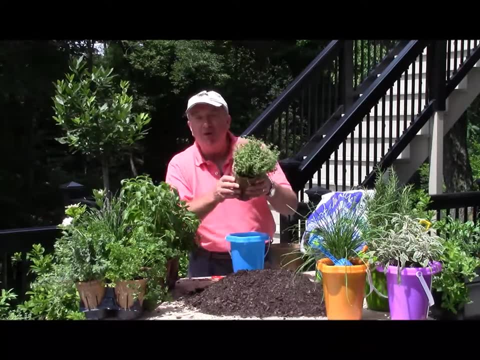 there's no waste, there's no plastic to recycle and they get away to a very quick start. Very important for children, because they tend to be a little impatient, aren't they? Anyway, when you start off with these, as you see, you get nice, good, big, strong plants that are, of course, sustainably. 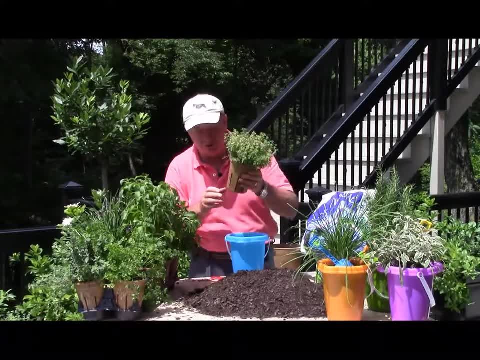 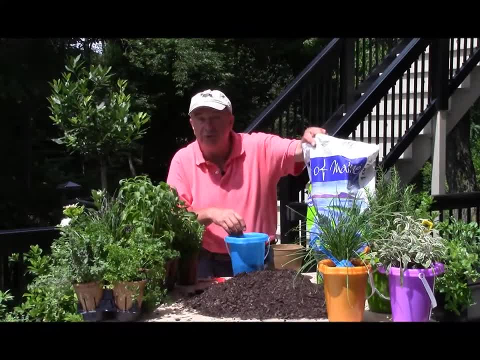 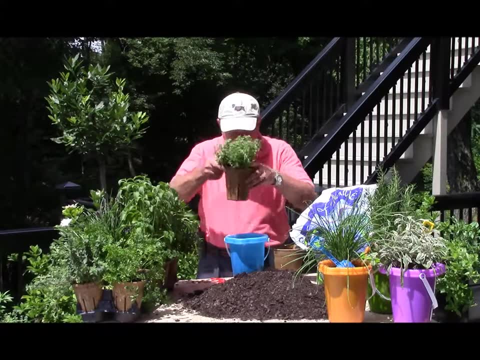 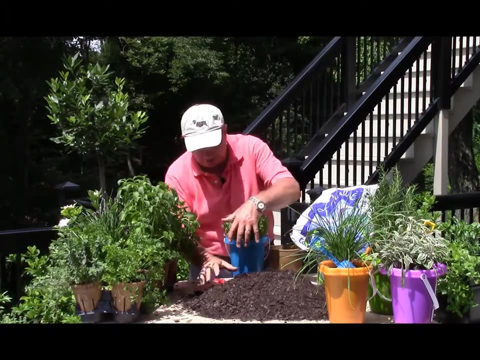 little bucket with some compost- and here I'm using Coast of Maine lobster compost. here I like the fact that this is approved for organic purposes- Then take your plant and just put it in the middle of the little bucket, Push it down a little bit so that there's a little space left for watering. 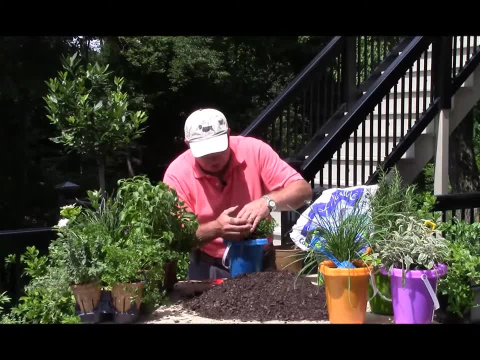 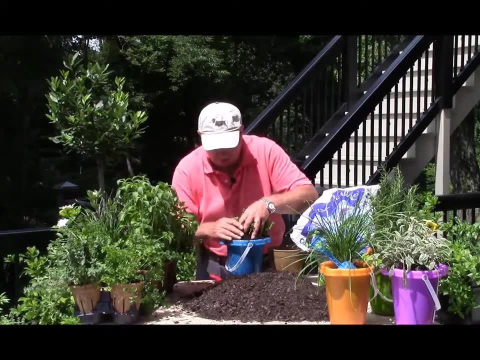 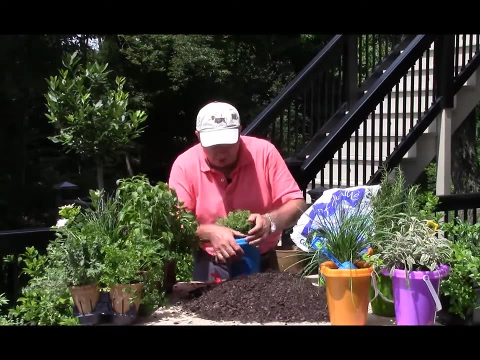 and then simply just fill in with the compost around the side, making sure that you've got good contact with the sides of the pot, because that's where the roots are going to come out and the compost. So just fill that in like so and in no time at all, as you see, you've. 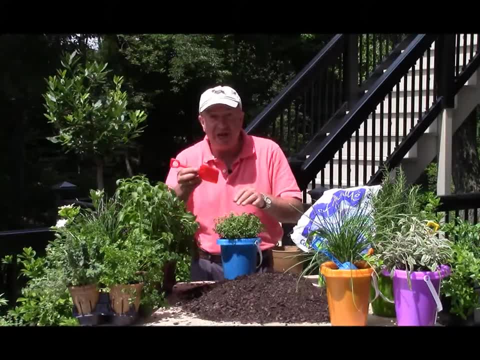 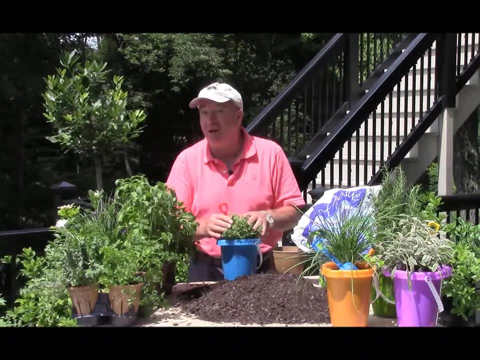 got a herb that's very attractive and pretty. You can take their name, if you wish, and put it on the side of the little, the little spade here, so that this is individualized for the various children. Now I'm using here lemon scented thyme. 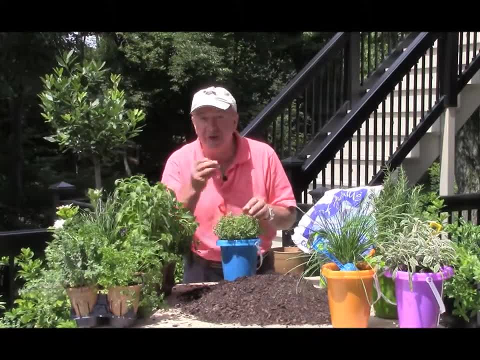 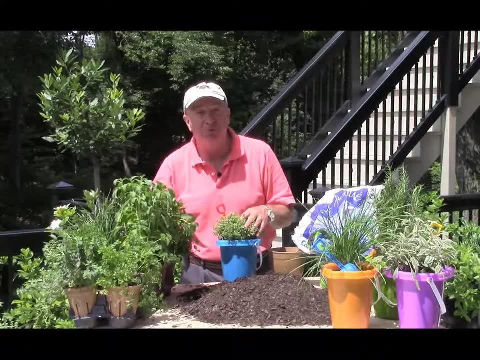 Which, of course, is absolutely gorgeous when you just touch it and then smell your fingers, and great to eat too. In fact, there's lots of varieties that come with these edible plants, from Footprints Plants, and if you watch in Jonathan Bozak, I'm sure will be giving you all sorts of 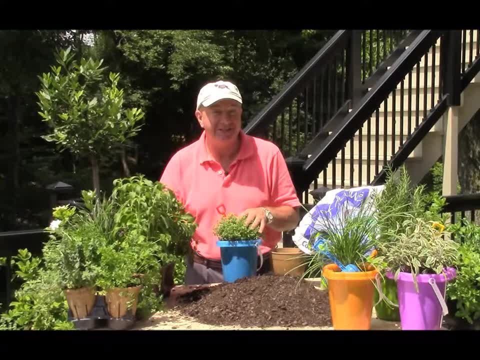 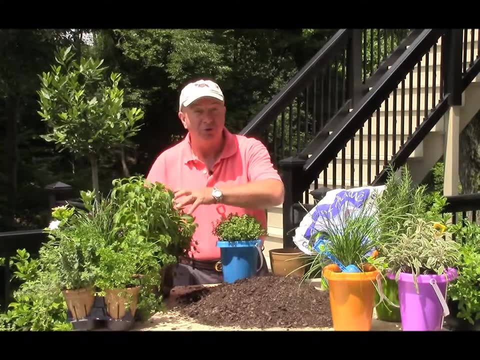 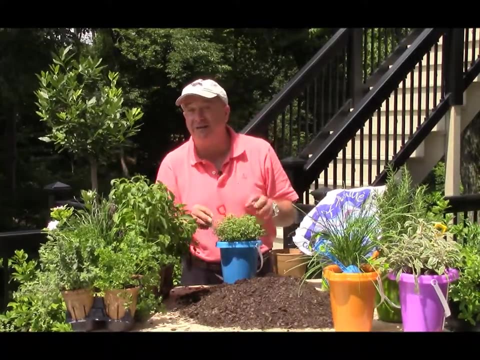 ideas that you can use them in all sorts of very tasty and interesting recipes. Now the plants are available from a network of garden centers throughout the northeast and mid-Atlantic states. There's lots of different ones to choose from, so you can choose the ones that are likely.